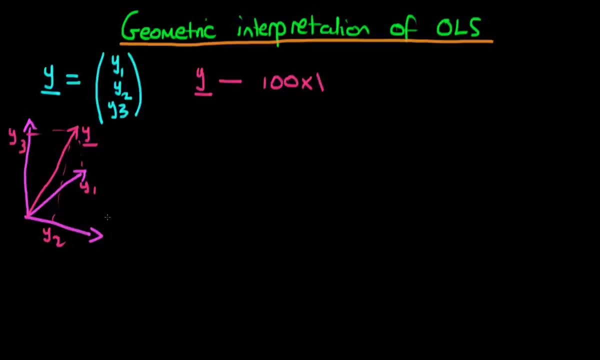 So we can't actually draw it using the three spatial coordinate axis, But we can still think about y as representing some sort of vector in a sort of higher order space, and we can draw it abstractly just as that. Furthermore, if we sort of think about our regression model, So our 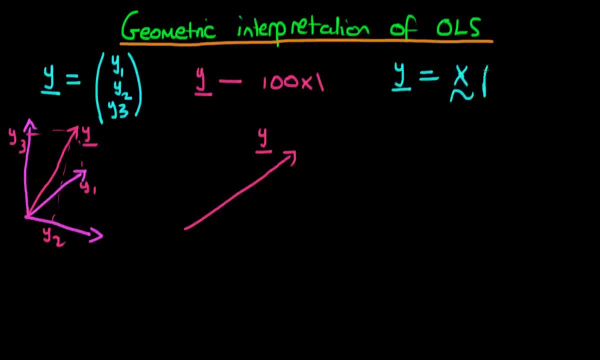 regression model is: y is equal to x times beta plus u. And we can think about that and we can about x. here we know x is our matrix of our independent variables And we know that we can sort of think about each of the respective columns as representing the particular space. 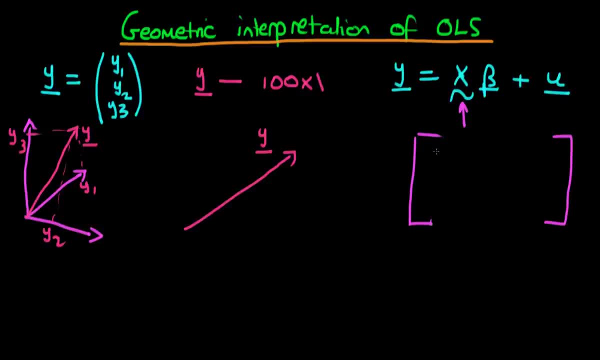 span by that independent variable. So typically when we're dealing with an OLS, the first column just contains one, because we're typically talking about having a constant in our model, And then the second column might represent the value of a variable, x one. So we have x one one as its first. 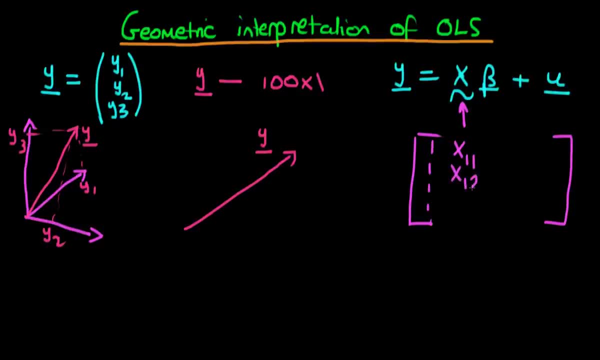 value for the first person, And then we have the second value of x, one for the second person, And then we have the third value and the fourth value respectively, And then we might have, let's say, another vector of observations for another variable, which I'm going to call x two we have 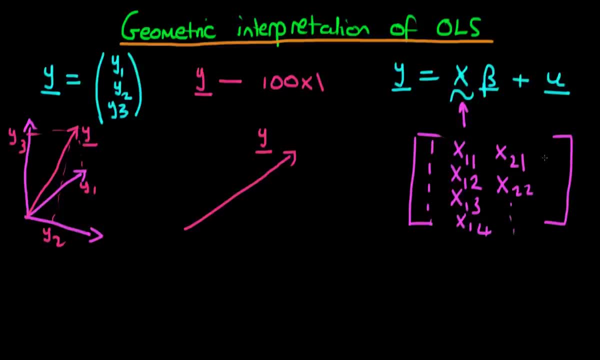 that for the first person, we have it for the second person, etc. And we can think about each of these respective columns As representing a particular vector, space. in other words, it's a vector in space. And if we were to essentially take each of these vectors, so we take the first vector, which is just a. 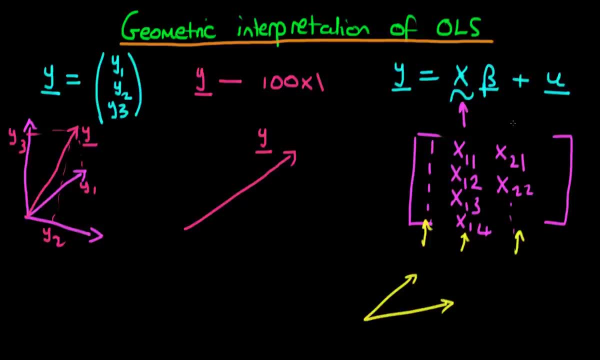 vector of ones. take the second vector, which is a vector of the second independent variable, and then the third vector, which is a vector of the third independent variable, then we can sort of think about the space which spans each of these three vectors as a sort of plane, because we 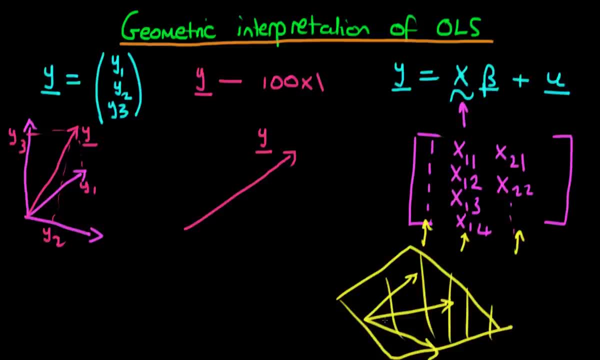 can sort of think about we're dealing in some higher dimensional space. And when we think about it like that, we can sort of think about what the purpose of ordinary least squares is, because what we're trying to do in ordinary least squares is we're trying to get as close to this dependent. 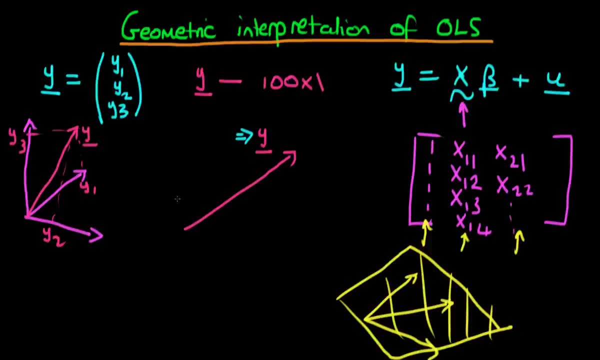 variable y or this dependent variable, vector y, given that we don't have a vector or a space which is as highly dimensional as the dependent variable. So we can think about the fact that we're trying to get close to y, even though 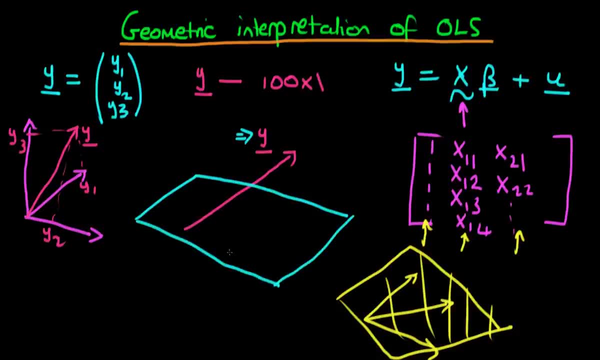 we aren't able to exactly get there. So we can think about the space which our sort of solutions got to be in as being represented by the column space of x, which is just this thing which I've illustrated here, And the idea with least squares is that we're trying to get as close to y as 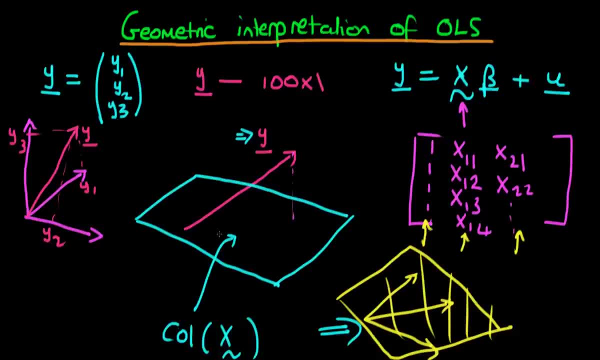 possible without actually leaving this plane here, because this plane we've got to lie on our plot. this plane here because we've only got so many independent variables, But we can get as close to y as possible on the plane And we can represent that sort of orthogonal. 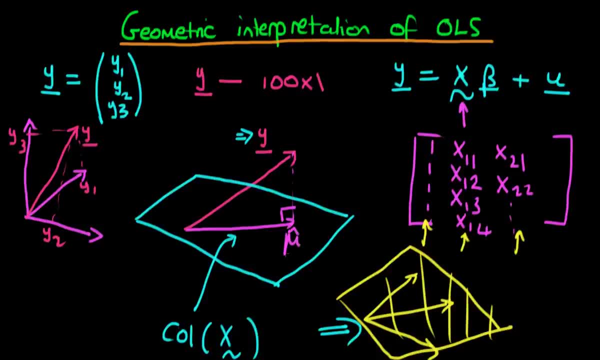 projection of y onto the plane by a vector which I'm going to call u hat, And because, essentially, what least squares does is, it minimises the square distance between u and y. essentially, we know that these two things are going to be orthogonal, which means that y minus u hat is. 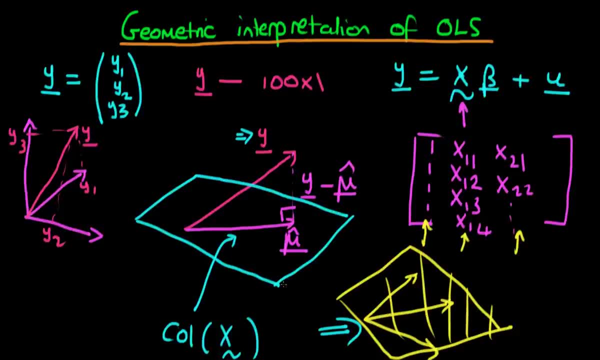 going to be orthogonal to the column space of x. So when we think about least squares in this manner, we can think about it as being composed of two steps. The first step is finding the orthogonal projection of y onto the actual space which is spanned by the independent 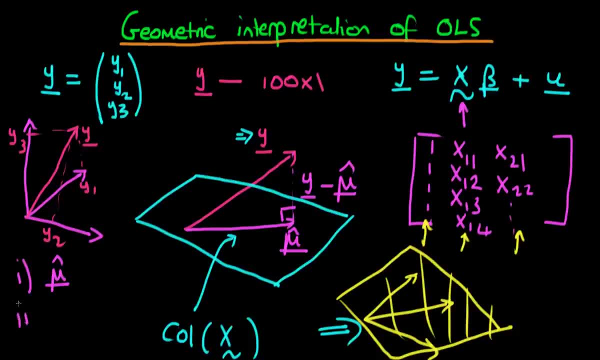 variables. So we're finding mu hat And then the second stage is decomposing mu hat into its various components. So it's going to have some component of the first dimension and some component of the second dimension of the independent variables and some component. 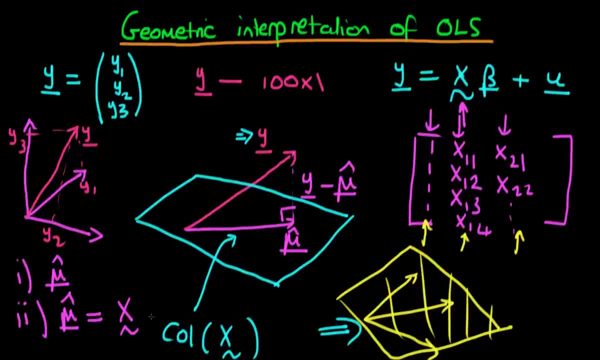 of the third dimension. So we can sort of represent mu hat by being equal to x hat, or, sorry, x times beta hat. And don't worry if you don't understand everything in this video. we're going to talk through a few examples in the next few videos, But I wanted to provide. 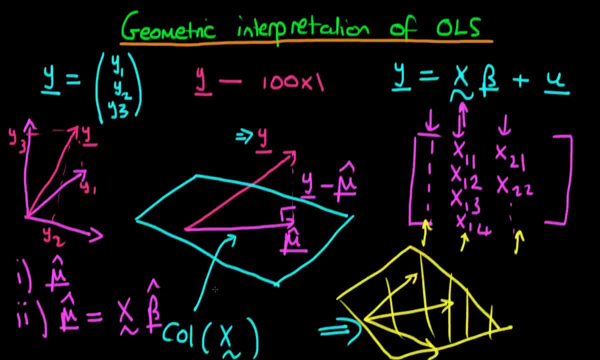 this as a sort of introduction to the geometric interpretation of least squares and the fact that we can think about least squares geometrically.